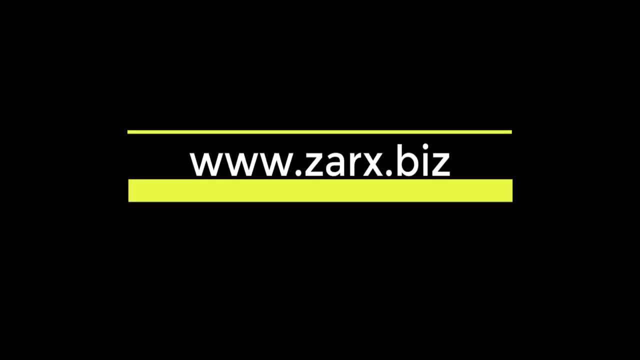 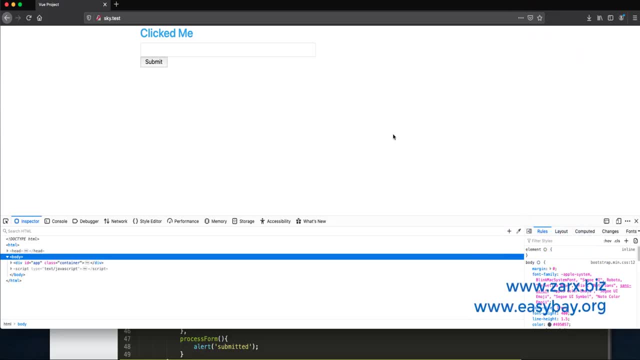 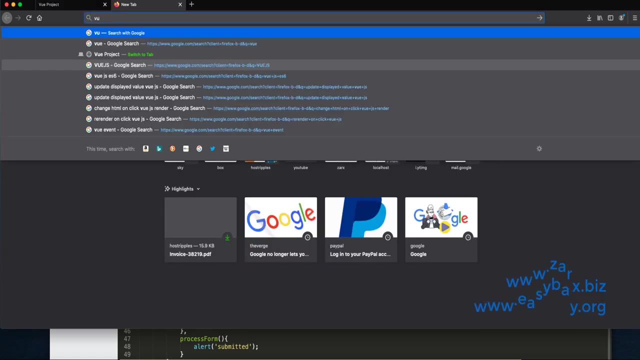 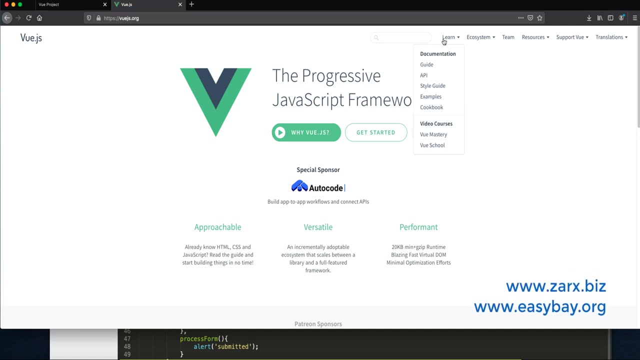 Welcome guys, Welcome to this brand new video of Vuejs. In this video we are going to talk about Vue directives. So if we go to the Vue website and there Vue directives are used widely, and if you go under Learn and API and on the left side, if you scroll, 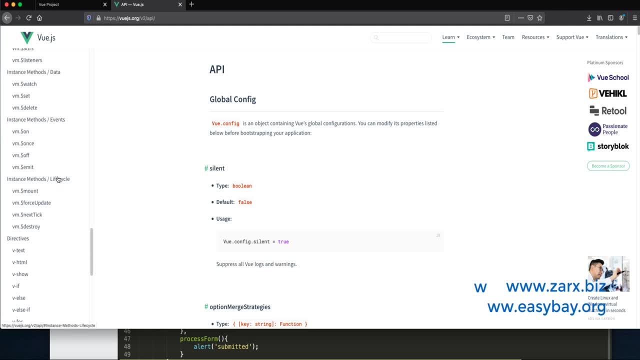 down. you should get the directive, the list of directives. So we have here these directives: the VText, VHTML, VShow. These are the very important directives used in Vue. We are going to be using these a lot and we already worked with the VOn, which works in Click. So now 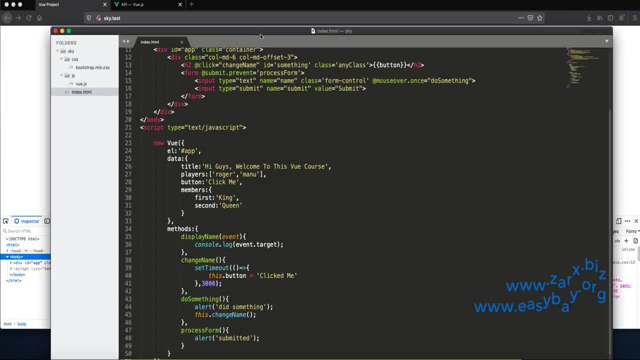 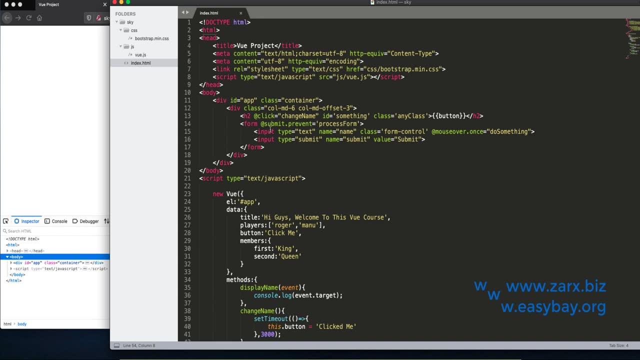 what I'm going to do. I'm going to remove some of this code that we were working here previously. So well, let's do that So you can see how to work with these directives. and we have this div and inside this div, we're working on In our 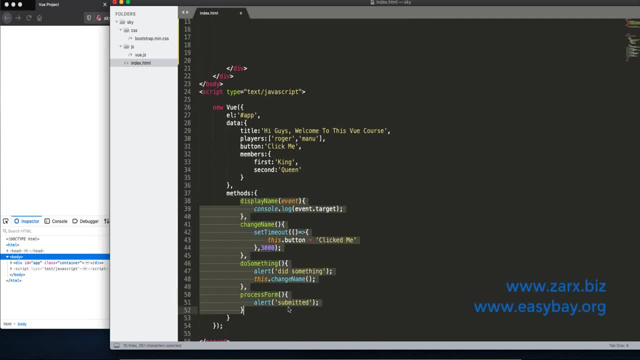 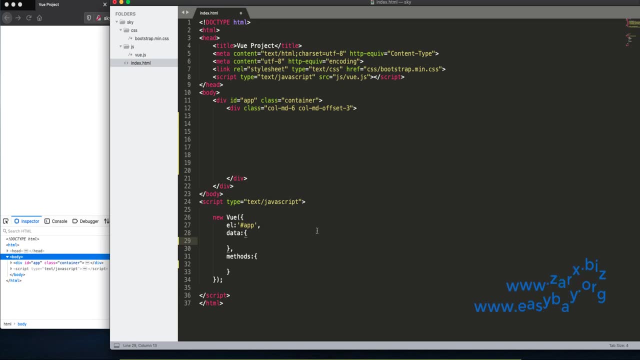 Vue instance. we don't need these methods. We can remove these methods and these properties. So we have just the blank method and the data object. So if I refresh the page it should be blank. We don't have any error. So the VText. 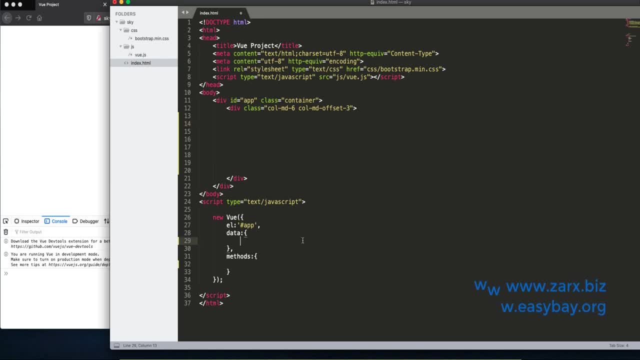 So what happens is that when we define any property, let's say, if I say a name property and I give it any name, like let's say Roger, and here if I say mustaches and then I say name, So it is going to find this name inside the Vue instance and it will print. 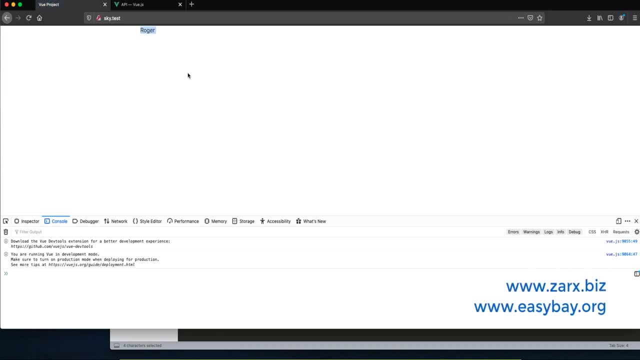 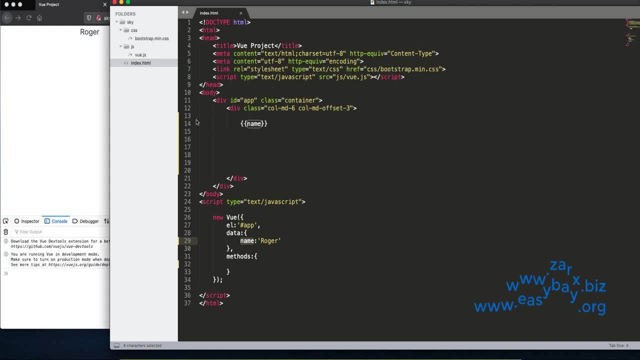 us the name, which is doing just fine. Now let me enlarge it for you. If in case we don't want to use it this way, we can also use VText. That's one of the other ways we can use it. So let's say you have HTML tag H2, and then you can say: 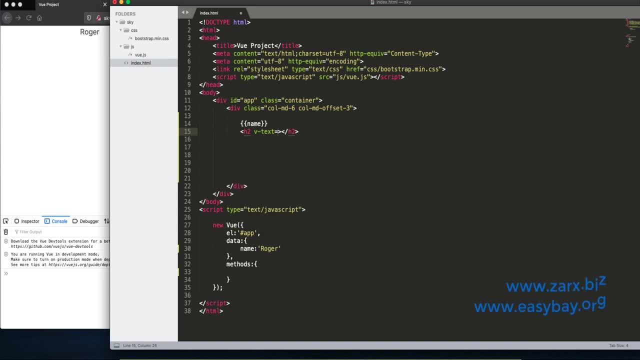 VText and inside VText. you do not need to put mustaches, You just need to put name. Now, VText knows that we are to look for, So it's going to do the same thing. It's going to print. and it's going to print the. 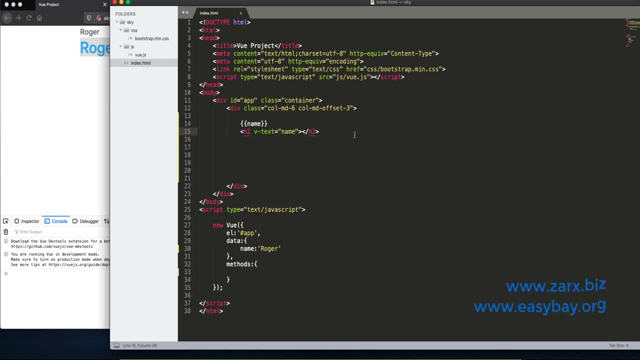 name. So if I refresh the page, we get Roger, So it takes from there. So here this is used this way. Either you can print this way or this way. that's up to you. Now the another directive we are going to use is the VHTML. Let me I have 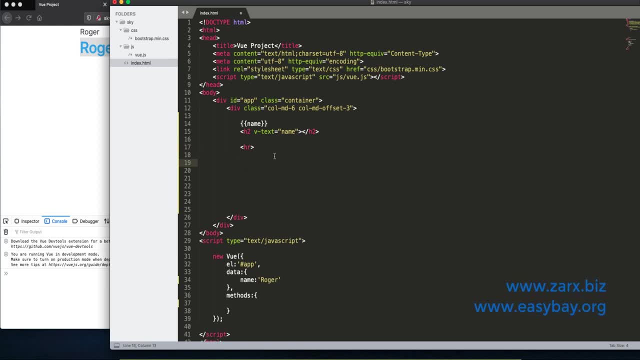 the HR2.. I'm just going to put a line there. So if I say H2, and the one that's going to be the HTML tag, so if I say H2, and the one that's going to be the HTML tag, 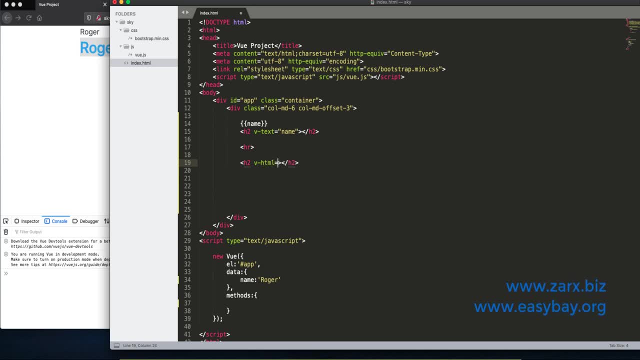 I'm just going to put a line there. So if I say H2, and the one that's going to be the HTML tag, I'm going to still get that right. I'm going to add the default bit: Volunteer Text. 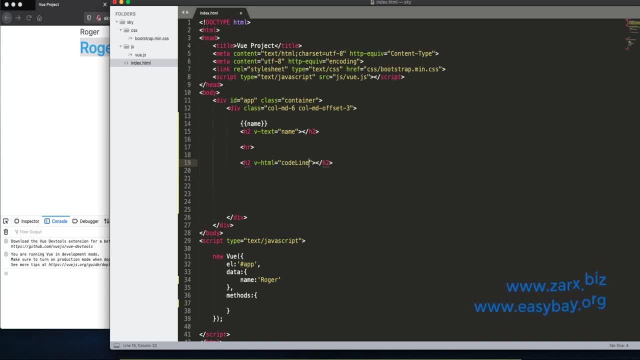 Now the next thing I want to do is I want to say vHTML and I say code line, code line. code line is going to be a property, just like the name, And the only difference going to be that we need to put some HTML in it. So if I say Dave, and I close that Dave And 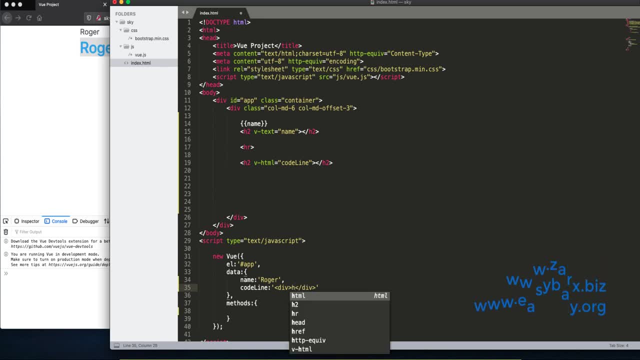 inside of the blade what I said here. I'm going to put a code line. Now if I close, I say it's H2 tag and then closing H2 and then from HTML and I save this. so it is going to remove these. it is going to render the HTML tags. that's the role of 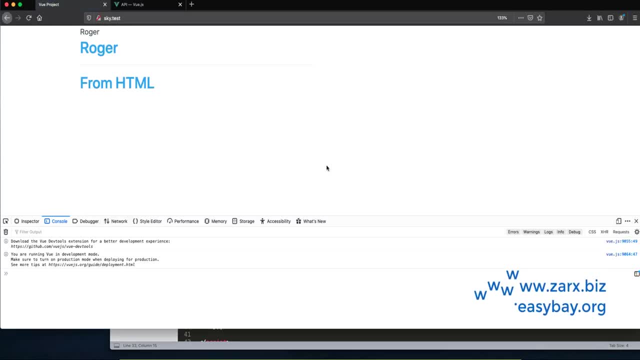 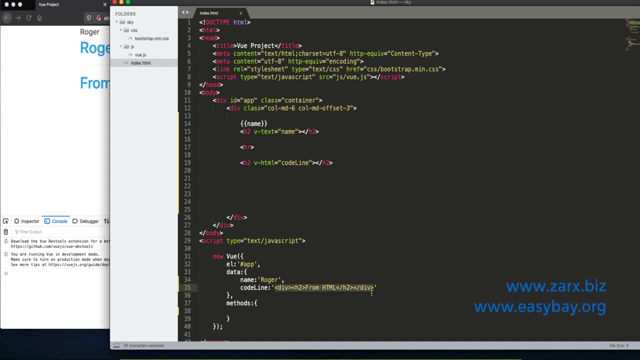 eHTML. so if we refresh, we get from HTML, and that's what you do when you pass HTML now. if you be using some code editors in your code in coming in the future, so you will be getting some content like this: so to remove the HTML tags, you can use VHTML. now. if you use V text instead of HTML, it will print. 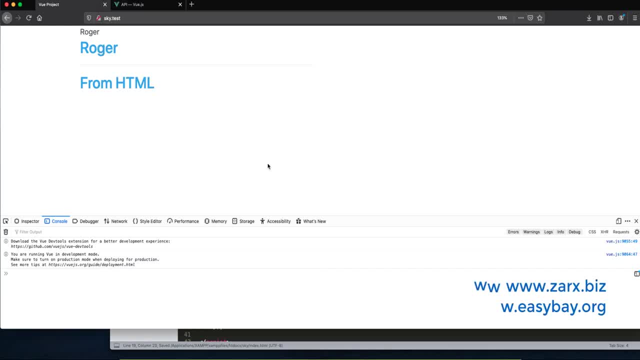 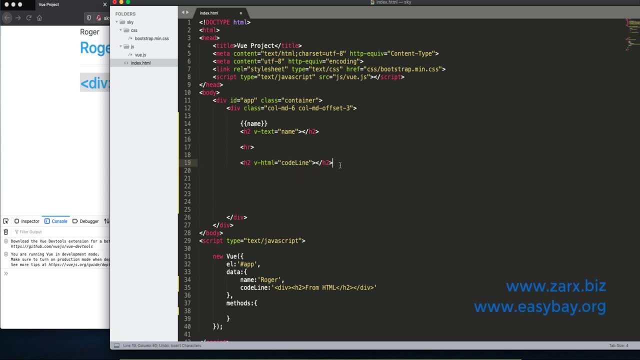 straight away. it will not render the HTML tags, so you will get the tags as well. so that's what VHTML does. so the another tag we use a lot is the we show, and it is quite simple. so what we do is: we say, we show, and whatever value you're going to provide here, it's going to be true, or? 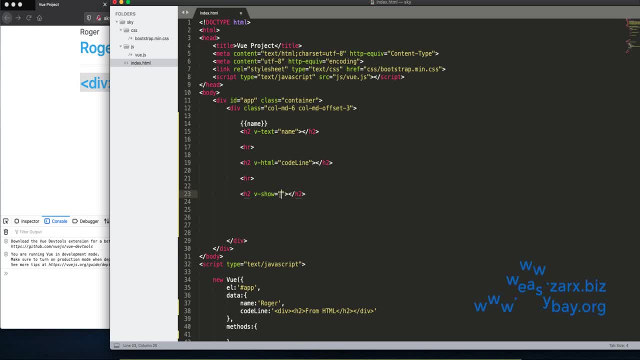 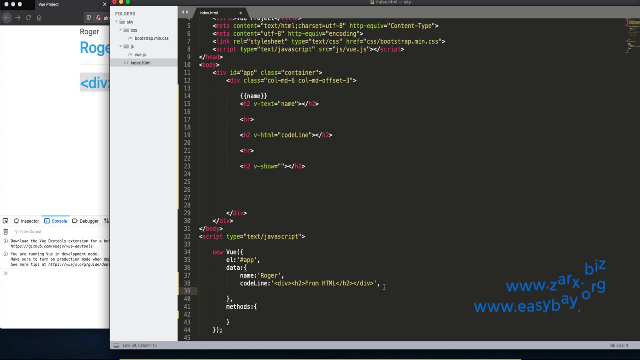 false. so if that value is true, we show or display the thing whatever is inside this HTML tag, and if it is false, it will not display it. so let's say, if I go into the properties here and I type here check and check is by default, let's say true. so if I say 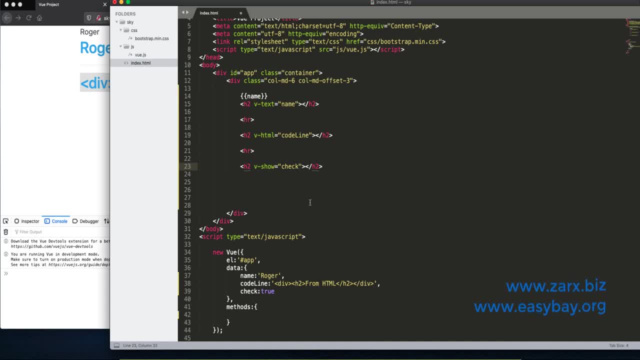 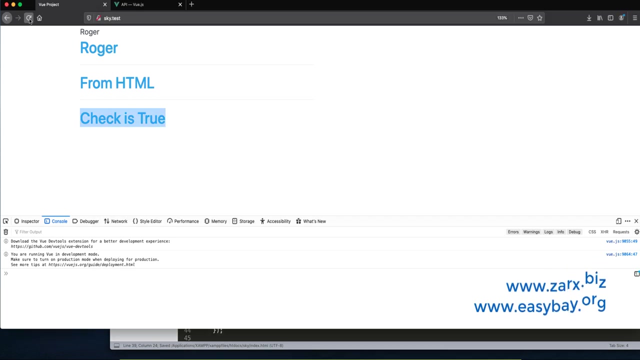 check in here and then I say: check is true, so it will print. check is true if in real check is true, which is true presently, so it should print. so we have check is true now. if you go here and you say false and then you refresh the page, it will not print because this check is false. 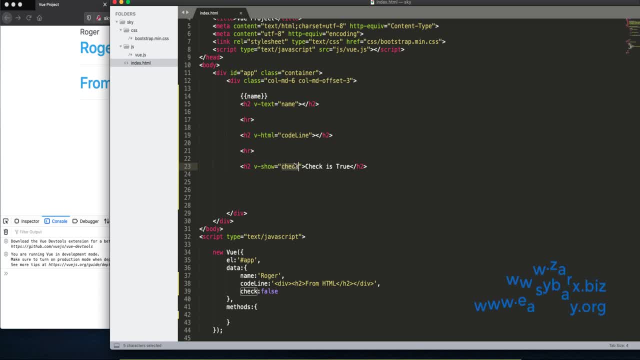 now and we show only displays if the value provided is true. so that's something it does it. you can put some condition or if you have some code in your function, you can set some value to true or false and can display accordingly. now a similar directive to we show is the: 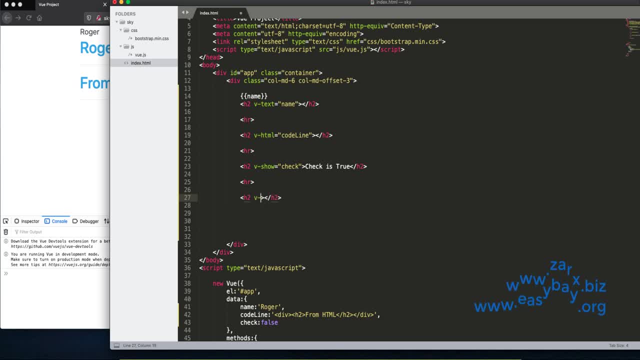 we if directive. it's quite simple. and we if is the if statement that we use, check if statement. so if I put check the same in here, it's saying they be if this check is true, the same way this show walks, it is looking for true and it is. 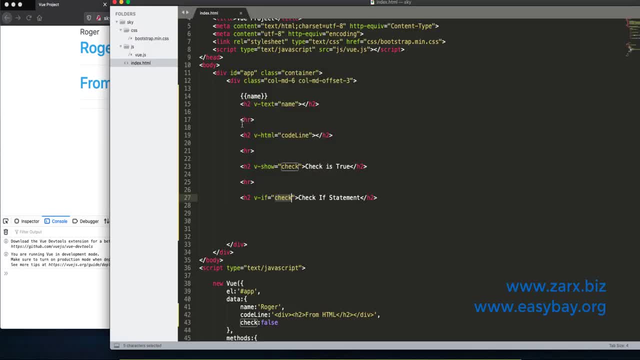 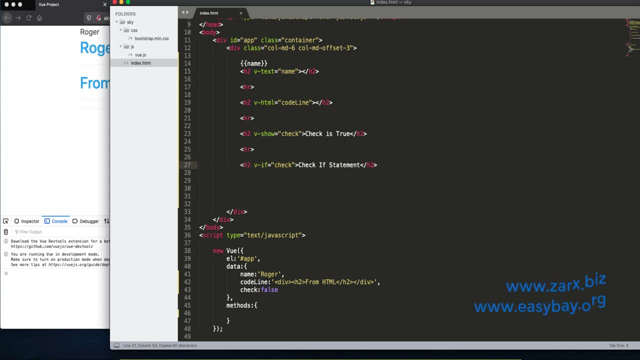 looking for true as well, so it shouldn't print for now. and it's not printing, and but if I say, if I just copy this line and here we can change it to else and we can say false, so now maybe true. yeah, it's in this case only one statement. 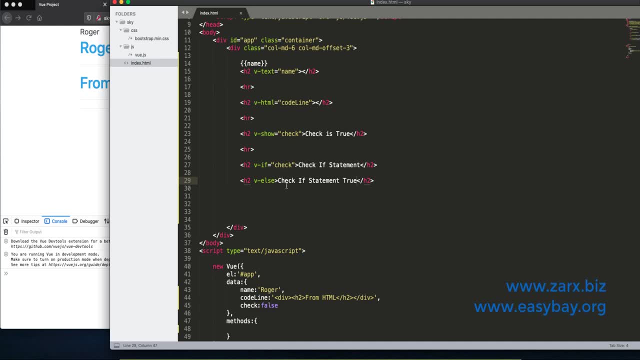 going to be fire. so check is false by default. so check is false by default so it will not fire. we will have check if statement true. so if I refresh, we get check if statement true and if I change to true it will fire the completely opposite line: check if statement. so the difference basically is we can use, we 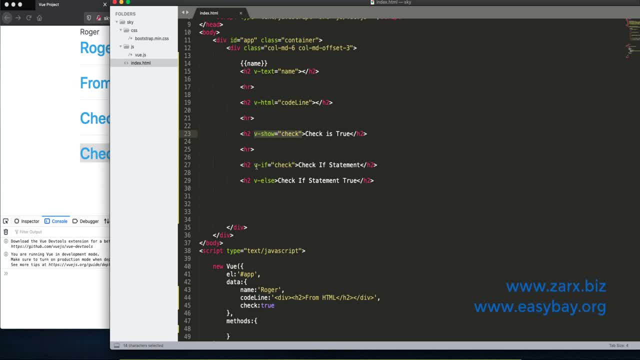 show to display or hide things, but we can. you all use we if and we else for more and wants to work. we can use it with the values. we can use we if and we else for more and wants to work. we can use it with the values. 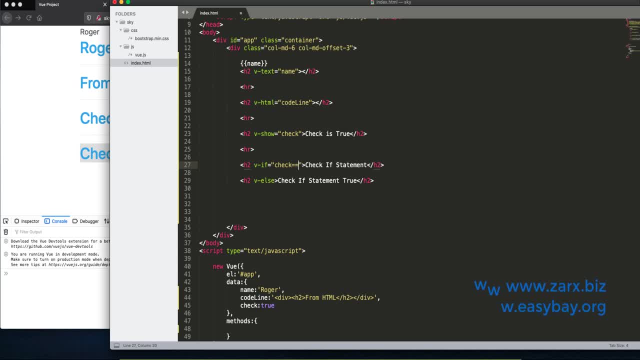 you can also check in here, like: if is equal to zero one, depending on the operation you're doing with the code. so we will be doing that in coming videos. now, the another directive I need to tell you about is be fine, and it's one of the. 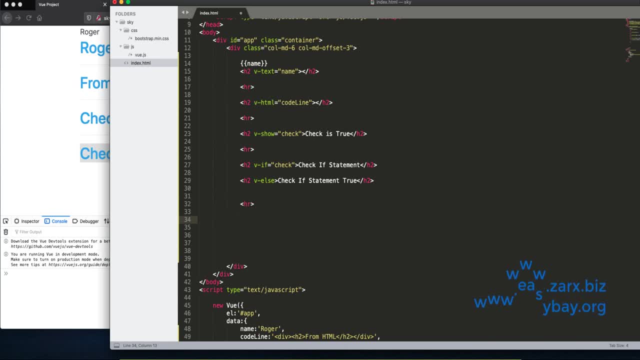 important directive in VJS. so let's say we have an image tag and we want to show an image. I'll give it a width of 300 and now, so, high up 300, now I want to provide it the property view property. so I say, let's say an image, now save this and let me add an image as well. an image. 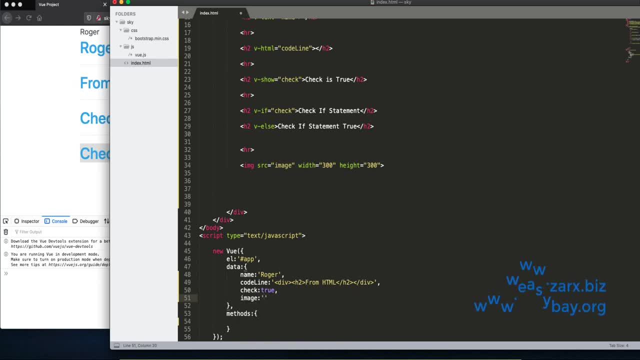 and we need to provide an image URL. so I have an image URL in me, so I'm going to copy that here and that goes right in. and that goes right in. we have two more images right there, okay, so if I go to the page and refresh it and inspect this, we get. 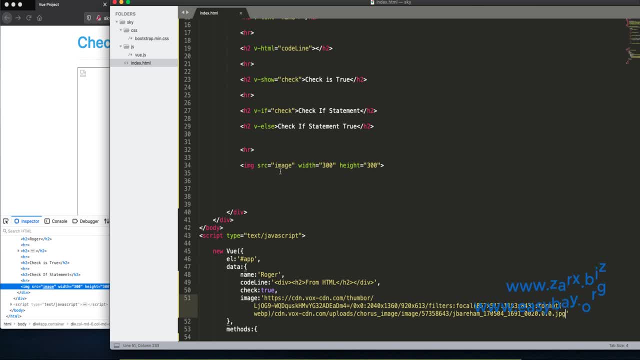 this text, only it doesn't know like what did. it means it's taking at the string, but we want to display the image URL. so what we do, we say we bind and what happens is it is going to bind and look for the text if it is present in view. 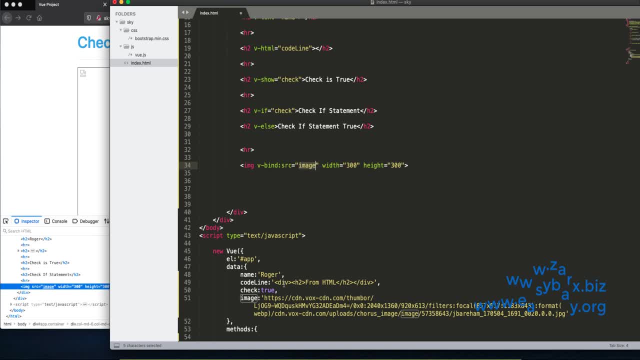 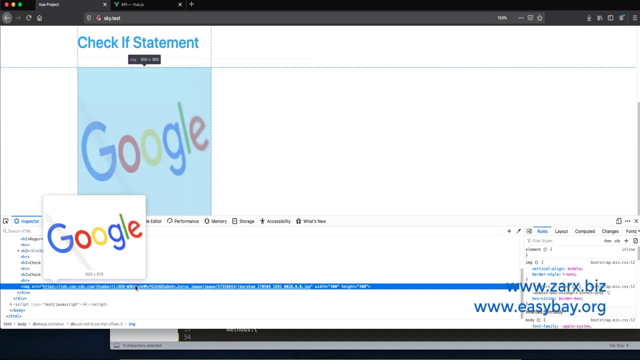 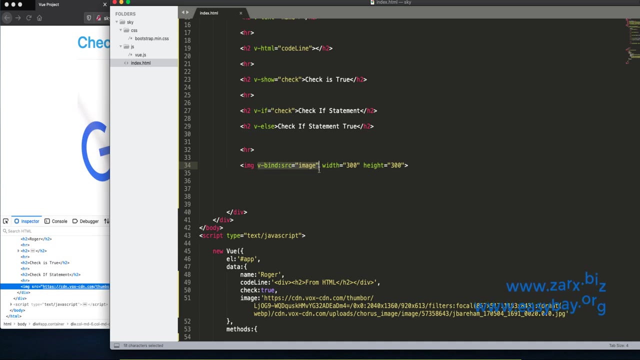 instance, as a property. so it is present in here and it is going to render it. save this and refresh the page. now we have the image and we have the URL as well. that's how you use it. now, the shorthand to work with be buying. you can. 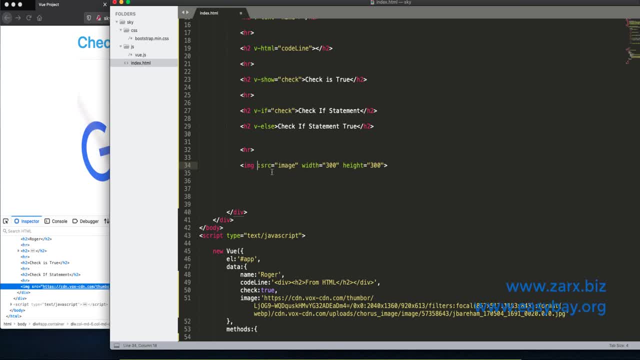 write it this way or you can remove this. we bind. you just have two columns and source and then you can refresh the page. it's still be walking. so this is one of the way using it. you can use it when you find, or just two columns, it's up to you how. 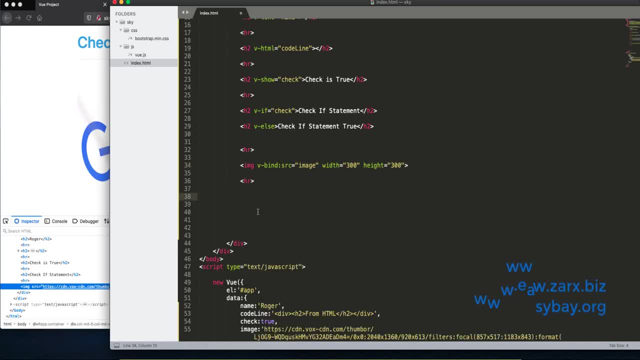 you want to do that movie model directed. we model directive is used in forms. so if I let me create a form in here for our inputs and I said we model and we model going to be, you can do any name to it. so I see title. so we create a object. 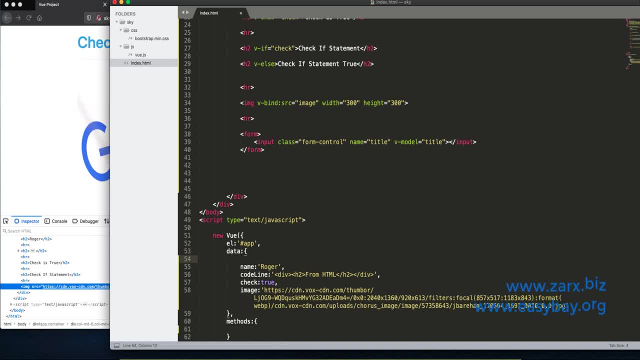 here for for the form to get the wellies from. so I say form and then an object and inside it I say title. now the title needs to be empty by default because the form field, we need to fill it and that then it's going to be assigned. so this title is going to be assigned from this. 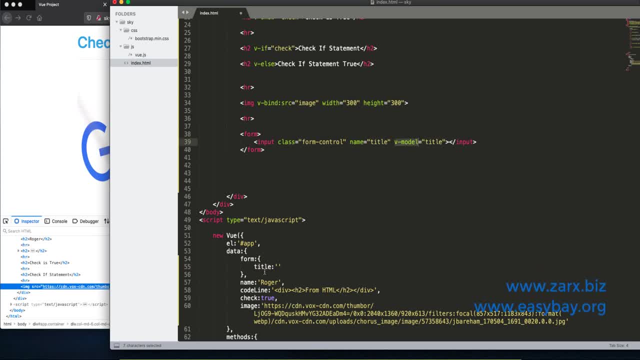 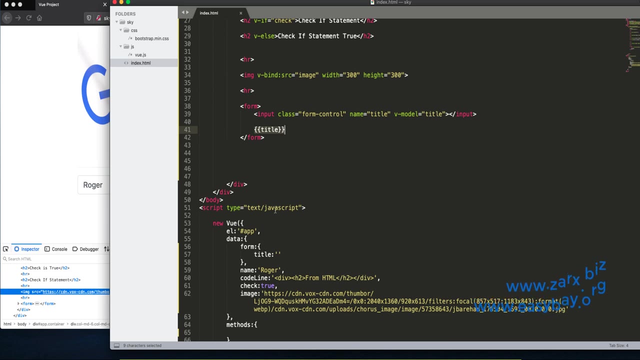 we model. anything user puts inside this input goes in there to see. to demonstrate it what I do. I put mustaches here and there. so if you save this title, ok, it is going to sign the title. but I made a mistake here because I created a, an object, and then the title we need to get. 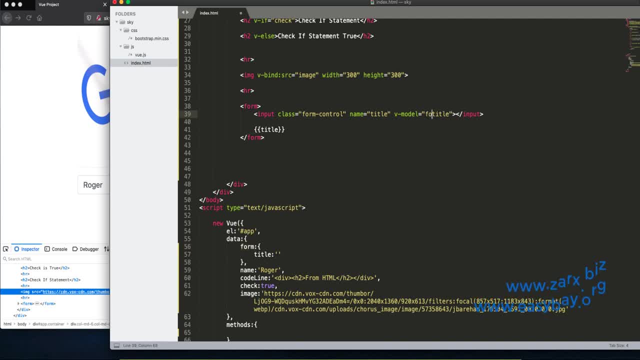 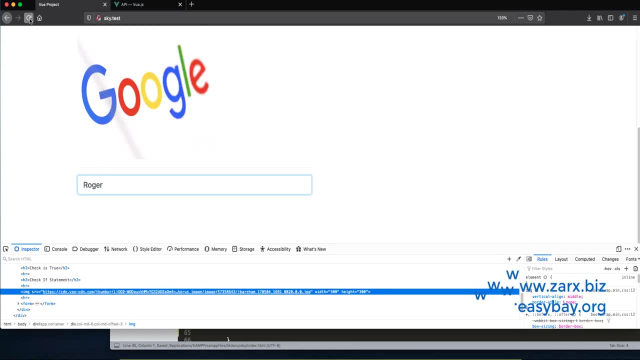 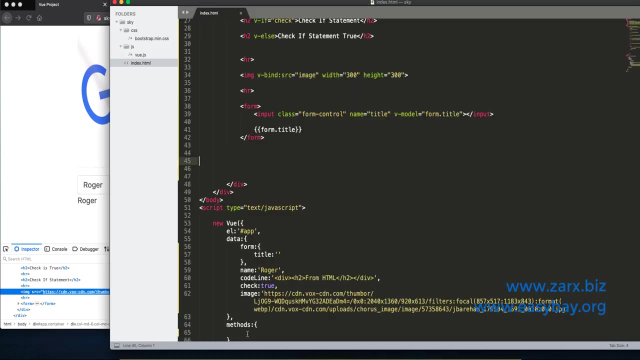 the object and then the title. so I need to say here formtitle and similarly we need to say formtitle in here. save that and refresh the page. if I say browser, you can see that I added value here and printed here and that's because I just added here that is assigning the value. 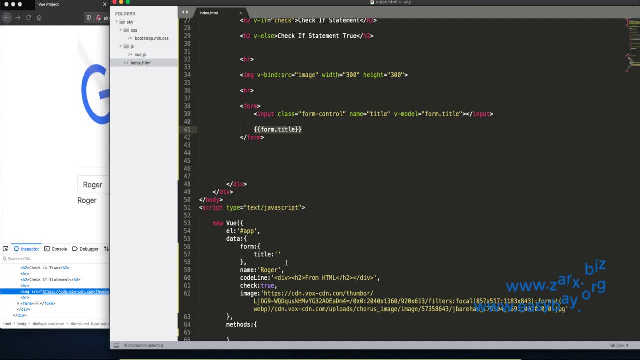 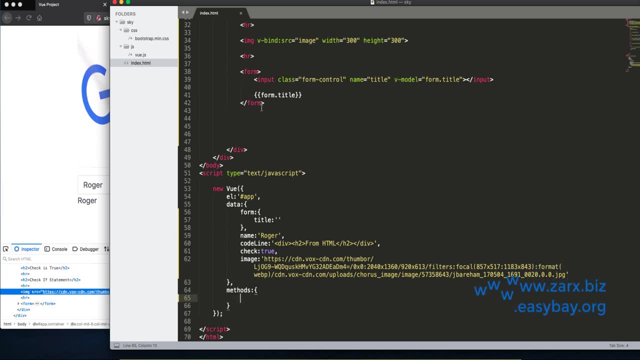 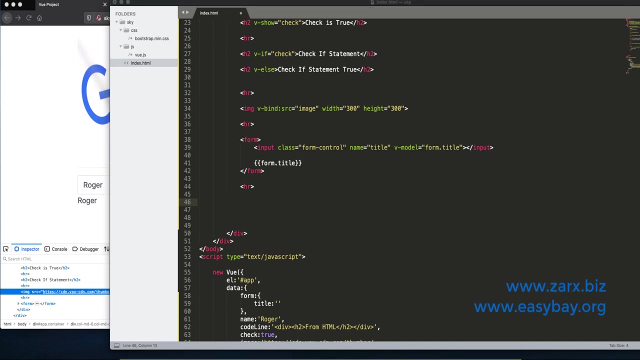 from the input to that particular property and you can use any function you can create in methods. you can use these values on submit of this form and then you can deal with the inputs in the way you and we deal with forms. so, in view how we deal with the for loop, this is the example, it's going to be the example. 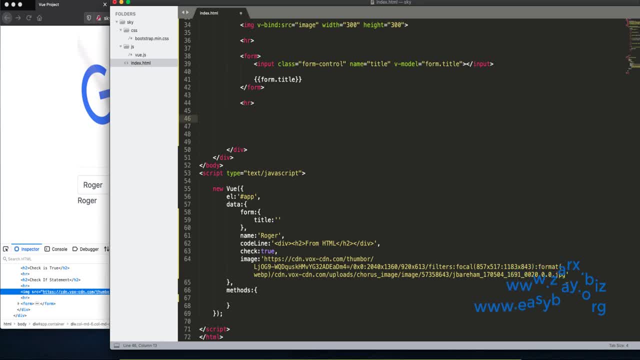 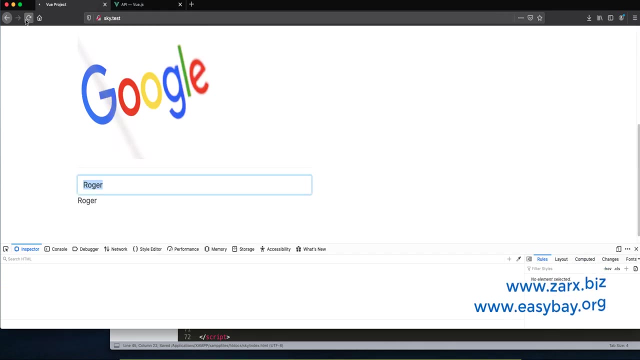 so I have an array of code, so what I do I add in here. so these are the players and the name of the players. so if I say that just print players, we will have the list of players here, but I want it in the one by one in ordered list. so, or? 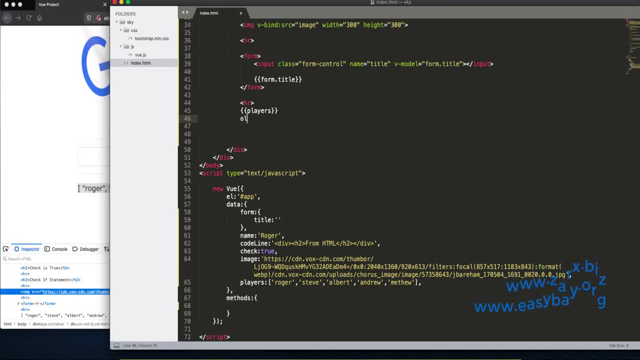 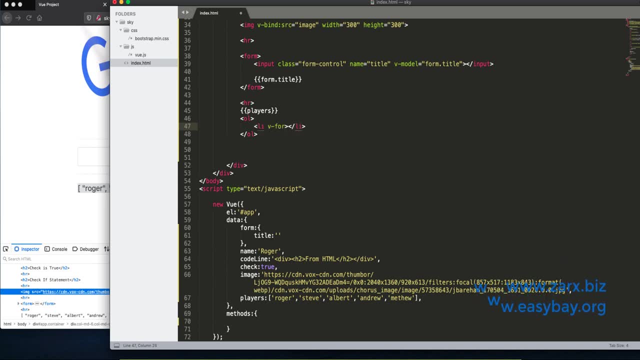 another list, whatever. so what I do is I say order list and then I say a like. now here I say be for, and syntax to use a for is that if you have an array of players, you will type that here in front of it. you can say anything. so I say I: 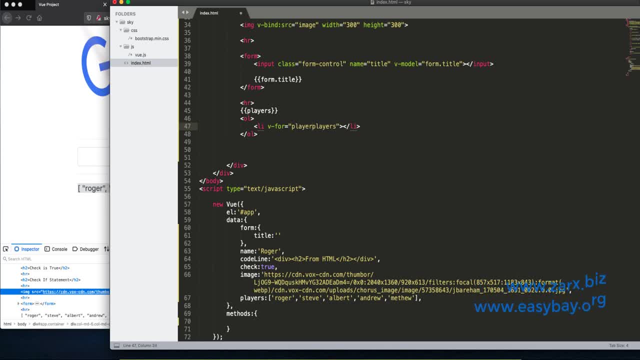 have multiple players as a player, because I want each time a single player in players. so player in players and in here I will say two mustaches and then player. so we are getting this player and I show and get here. now we need to get the index of these loop whenever he truly prints the head looking at view, quiet to. 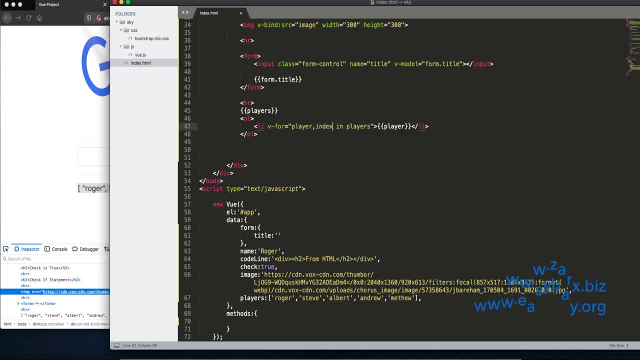 have indexed. so we'd say index and put this bracket and we assign this to the key. so this is the key and inside it would say the index. so this, each value have a key and it will assign an index value. so this is the vbind going on here. 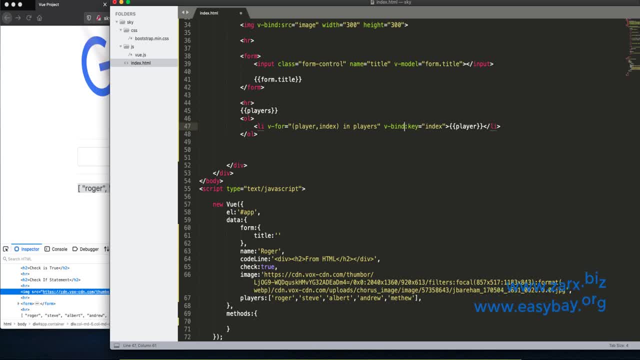 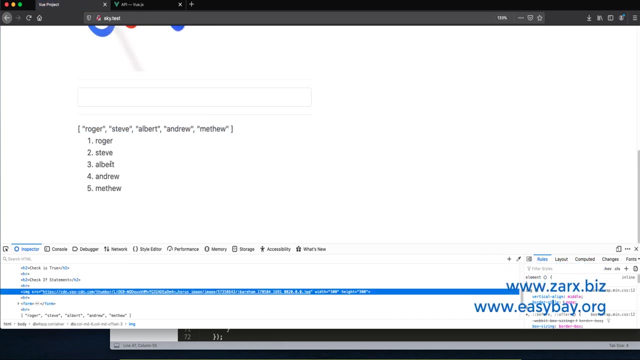 you can either say vbind, then colon, or just the two dots. it's totally up to you. I prefer this because it saves time. so I save this and I go and refresh here. you can see it printed: the name one, two, three, four, five. we have all. 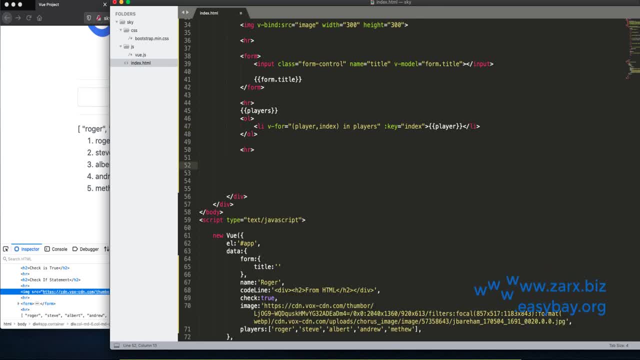 the names printed be on directive. so if I create a button on and then we say we on, we need to tell what to do. so we say click and we say do something. now, this do something is a function that we are defining here, so we need to go into the 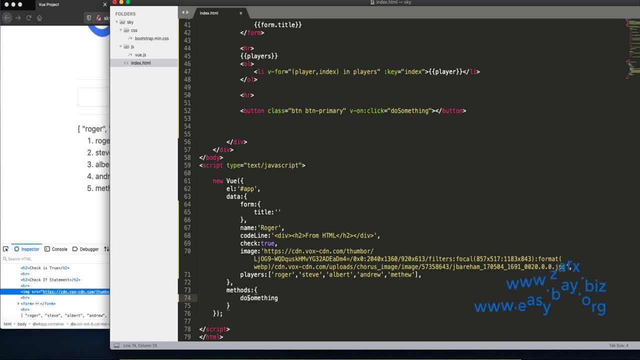 methods, methods, function is the same thing. so I just put here and this is how you define a method, and for now I just say alert, yeah, so on, click. I want this method to work. so if I refresh the page we have a button text in the button. if I click there it says yeah, now we can even say that like 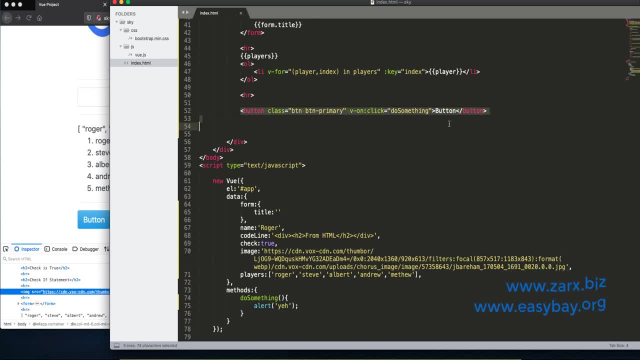 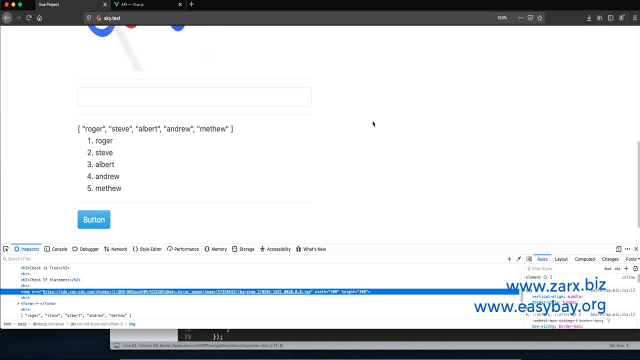 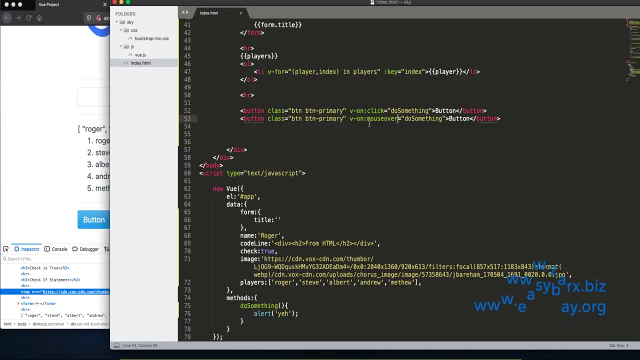 instead of click. we can have more events on this one. you can say: mouse over, it works like hover effect. so in first one it will work on click and in this one it will work on hover. so this is how you use it instead of using we on and. 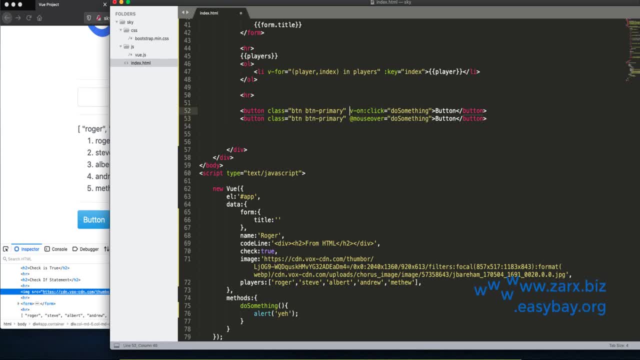 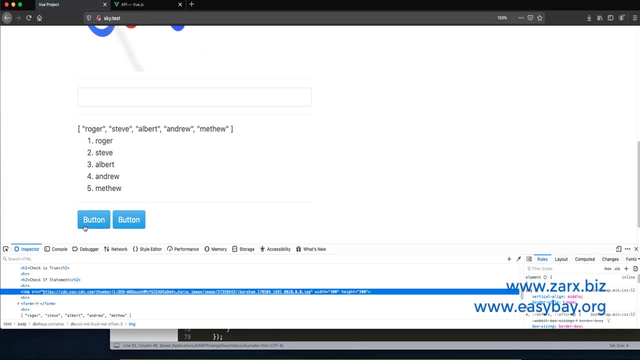 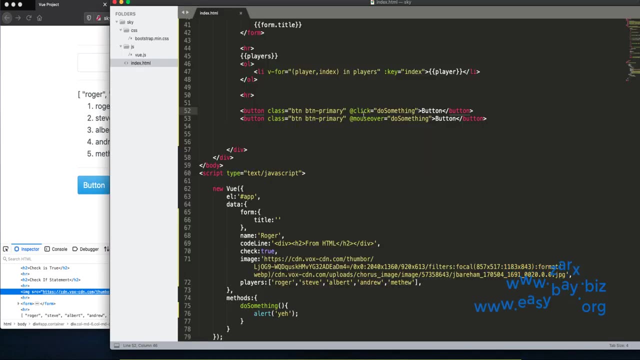 the shorthand will be the at. you can replace we on with at, and it will work the same way. so if I refresh the page and click here, it still gives me the yeah and here yeah again. so this is how you work with the view directives, and these are the most used to view directives. you: 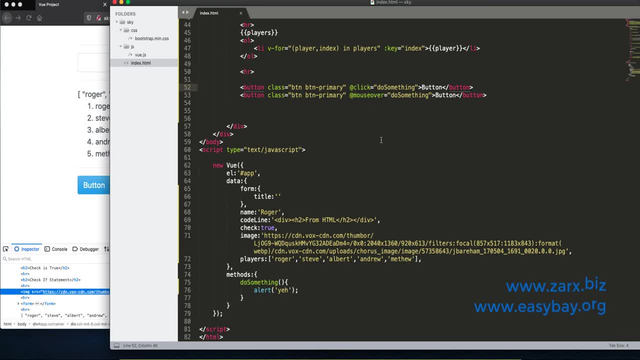 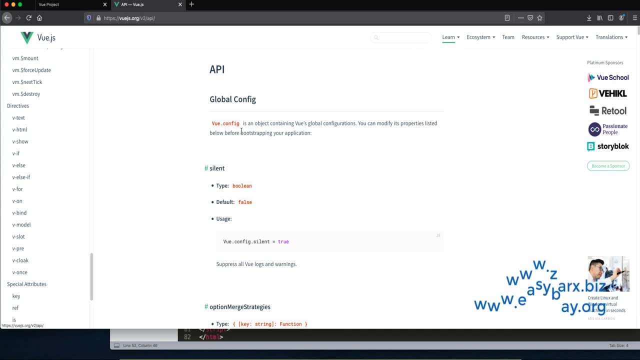 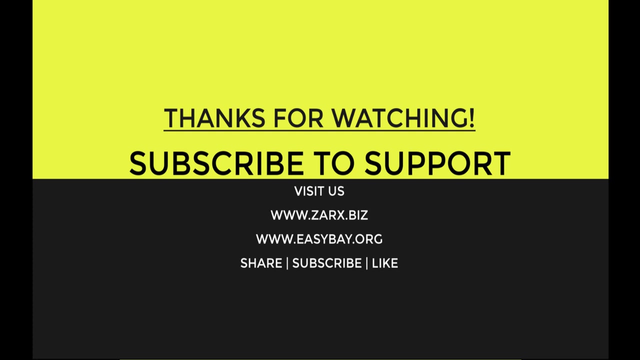 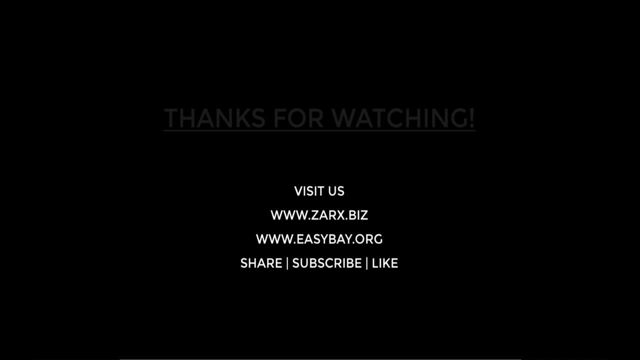 will be seeing. I will add this code for you and you can check that, and I advise you to go to this website, go under learn an API and look for view, directives and practice. if you liked the video, do subscribe and share. goodbye. thank you so much for watching and I will see you in the next video, bye, bye.